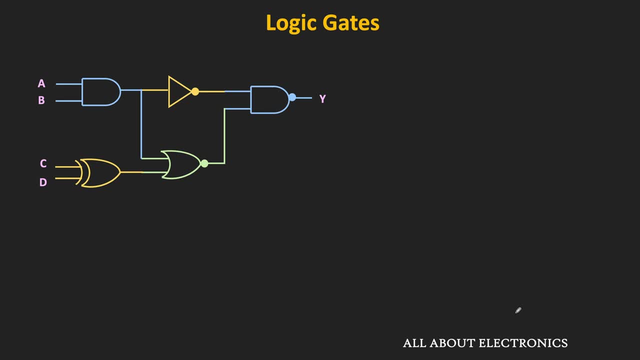 So these logic operations which is performed by this circuit, can be represented using the Boolean expressions Or other way around. if we have some Boolean expression, then it can also be implemented using these logic gates. So in digital electronics, when we are using these logic gates, then actually we are also. 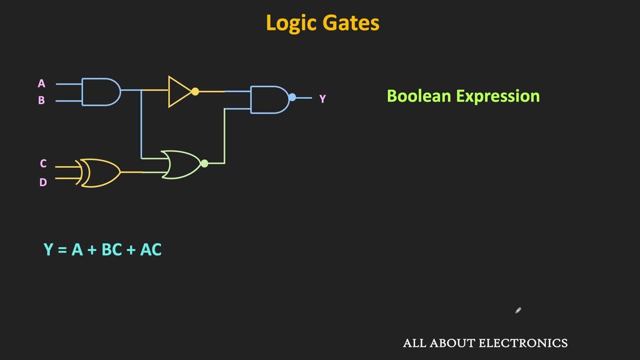 dealing with these Boolean expressions And therefore it is good to know about some Boolean laws, Because using these Boolean laws, it is possible to minimize the Boolean expressions. And if we can reduce the Boolean expression, then the number of gates, which is the number 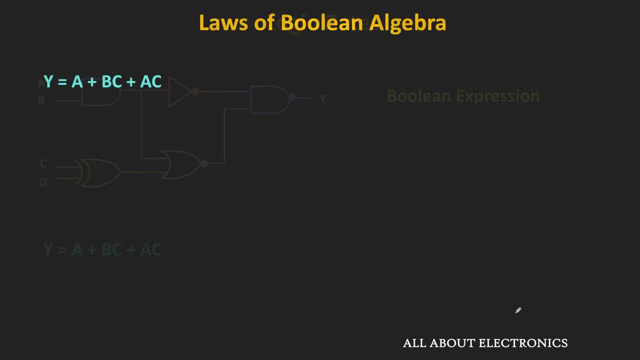 of gates required to implement that expression will also reduce. For example, if we know the Boolean algebra, then this Boolean expression is equivalent to a plus bc. So that is why it is good to know about the Boolean laws. So here is the list of some Boolean laws. 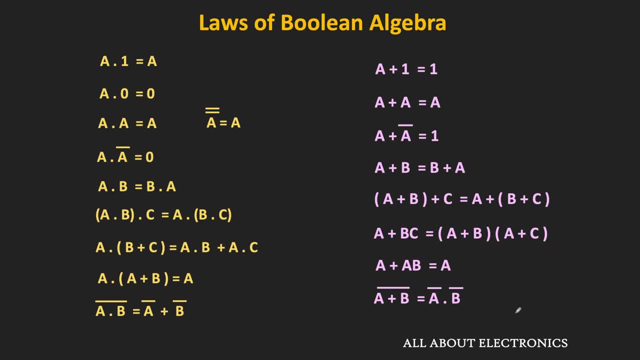 So most of them are pretty straightforward to understand And all these laws can be proved using the truth table. So one by one, let us understand them. So first one is this: a.0 is equal to 0. That means the AND operation of this a and 0 is equal to 0. 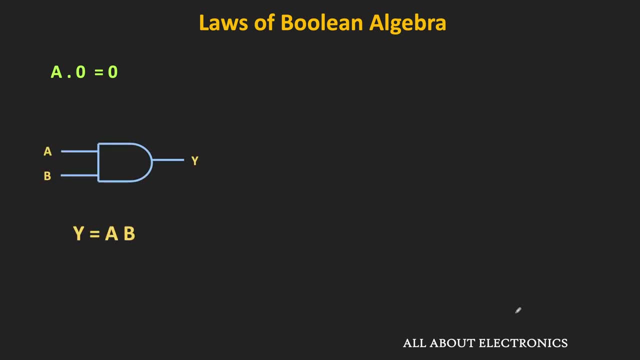 So we already know about the two-input AND gate And here is the truth table of the two-input AND gate. So, as we know, for the AND gate, when one of the inputs is 0, then the output is also 0.. 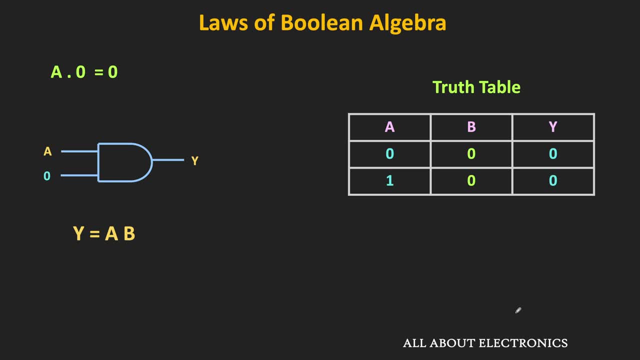 So in this case this input b is equal to 0.. So in this case, since one of the inputs is also 0, then the price sur deliverance is只 0.. always 0, so output will also become 0. That means the end operation of this a and 0 is. 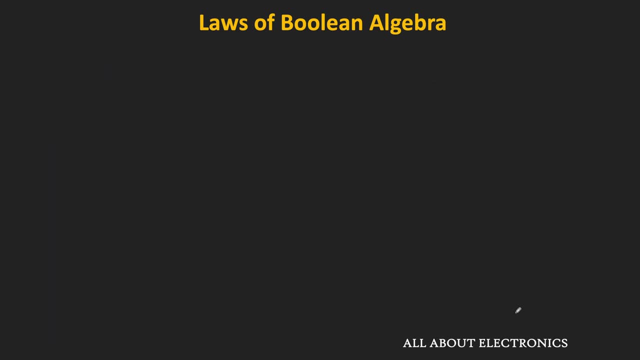 equal to 0.. Then the second is this: a.1 is equal to a. That means when we do the end operation of this a and the logic 1,, then the output is equal to a. So it is quite similar to our normal algebra. But to understand it more clearly once again, let us see the truth. 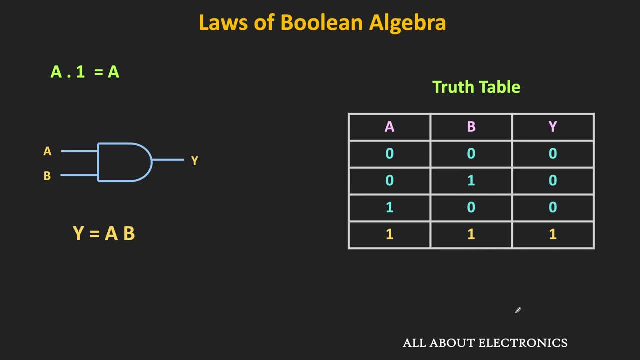 table of the AND gate. So in this case one of the inputs is always set to 1.. So here for the second input, a, we have only two possibilities. So when a is equal to 0, then the output of this AND gate is equal to 0. And when a is equal to 1, then the both inputs are 1. That 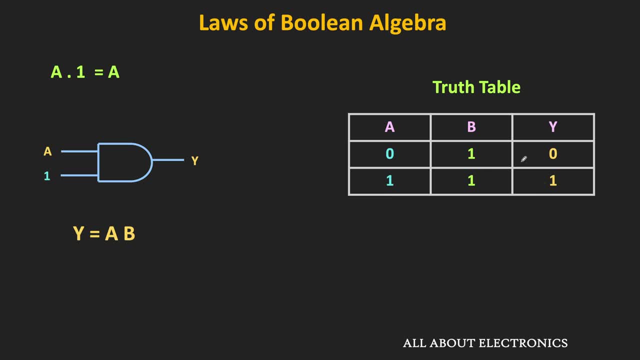 means in that case the output will be equal to 1.. So, as you can see, this y column is same as the a And therefore we can say that. So, as you can see, this y column is same as the a And therefore we can say that. 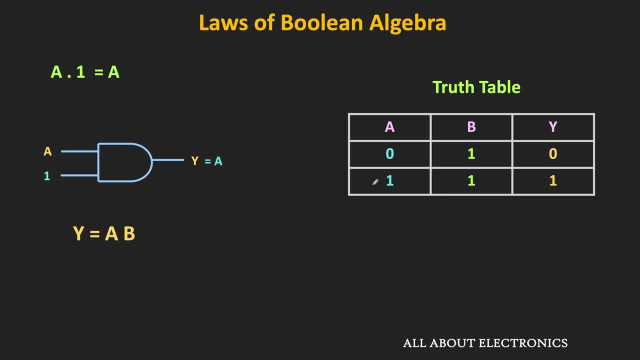 this: a.1 is equal to a, Then the next is the end operation of a and a is equal to a. That means during the end operation, when both inputs are same, then the output is same as the input. So this is the truth table of the two, input AND gate, And whenever both, 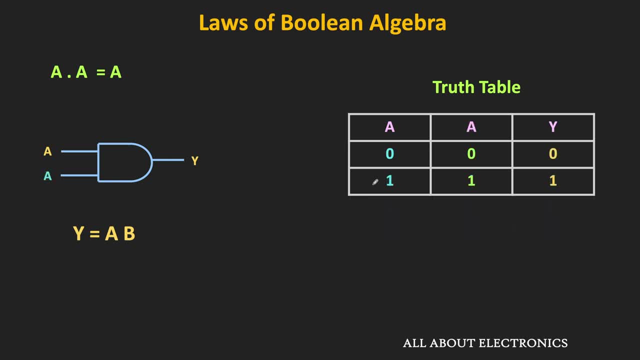 inputs are same, then this b is also equal to a. So in this case, for the input a there are two possibilities. So when this a is equal to 0, then both inputs are 0. And in that case the output of the AND gate will be equal. 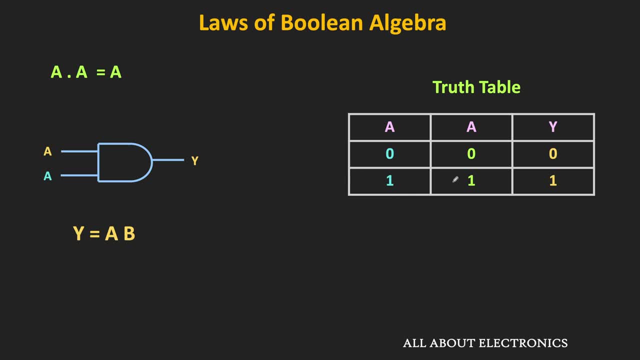 to 0. And when a is equal to 1, then the both inputs are 1.. Therefore, the output of the AND gate will be equal to 1.. So, as you can see, this output, y is following the input. That means this y is equal to a, And this is also true when there are more than 2 inputs. 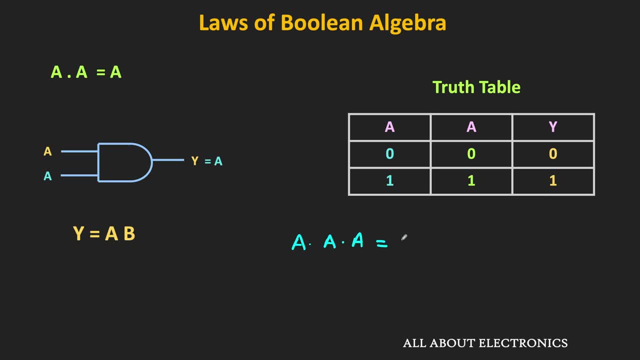 So whenever aaa, then that is also equal to a. Then the next is the end operation of the a and the a bar is equal to 0. Where this a bar is the complement of the a. So to prove that once again, let us see the truth. table of the AND gate. So in this case this: 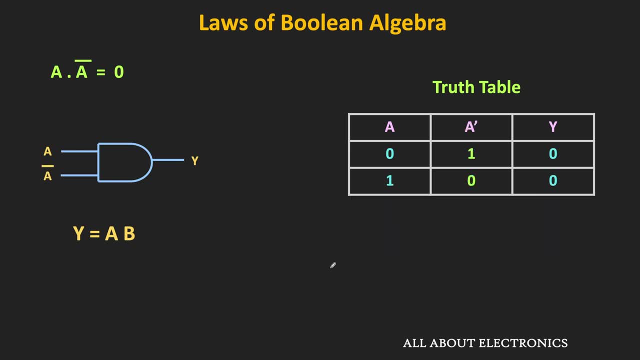 second input b is equal to a bar. So once again for the input a, there are two possibilities. That means whenever this a is 0, then the input a is equal to a. So in this case this second input b is equal to a bar. So once again for the input a, there are two possibilities. 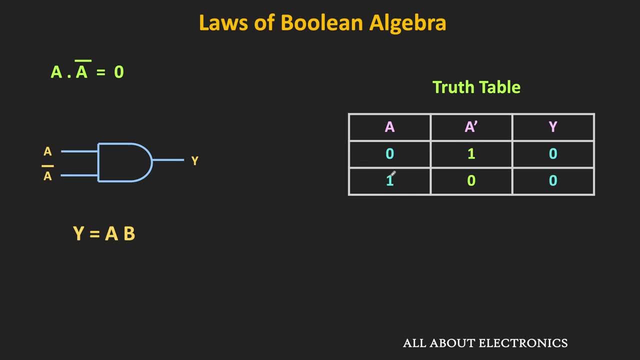 then this A bar will be equal to 1.. And similarly, when this A is 1,, then this A bar is equal to 0. Because this A bar is the complement of the A. So, as you can see, in any case, one of the inputs of the AND gate is always 0. 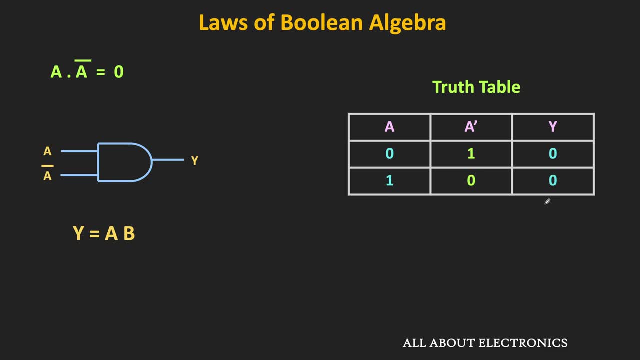 And therefore the output of the AND gate will always remain 0. That means this Y is equal to 0. And that is why the AND operation of this AND bar is equal to 0.. So these were some of the Boolean laws related to AND operation. 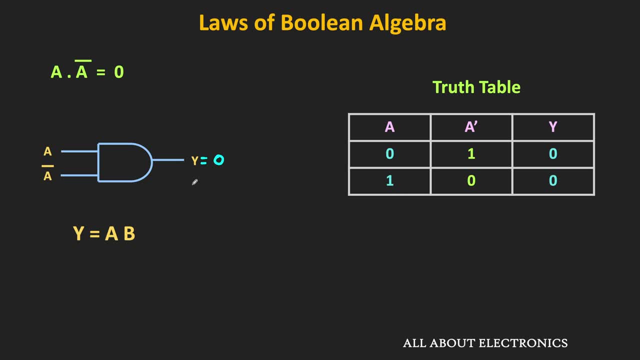 Similarly, let us see the Boolean laws related to OR operation. So the first is the A plus 0 is equal to A. That means the OR operation of the AND logic 0 is equal to A, And this expression is quite similar to our. 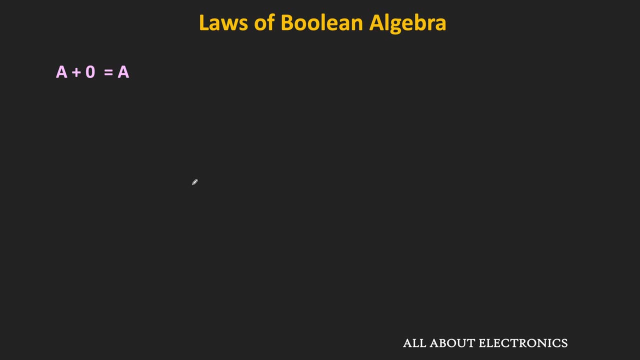 normal algebra. So to prove that once again, let us see the expression. So the first expression is the truth. table of the two-input OR gate. So for the OR operation, we know that when one of the input is 1, then the output is: 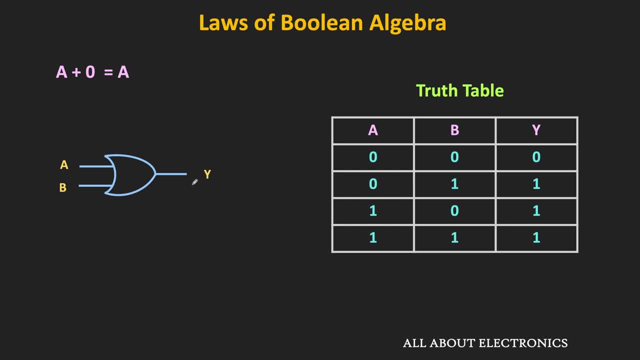 always equal to 1.. And when both inputs are 0, then and then only the output of the OR gate is equal to 0. So here, one of the input is always set to 0.. So now for the input A, there are only two possibilities. 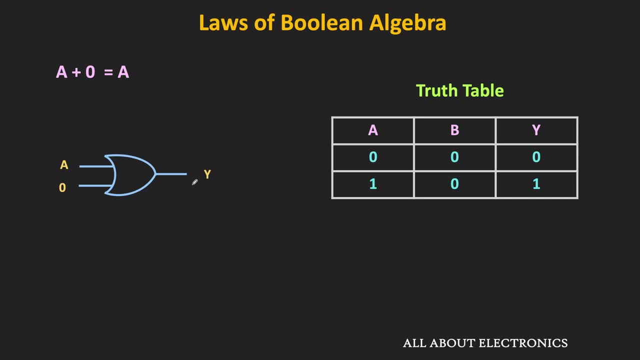 So, when this A is equal to 0, then both inputs are 0.. this output y is equal to 0. And when this a is equal to 1, then the output of this OR gate will be equal to 1.. So, as you can see, this output y is same as the a, So we can say that. 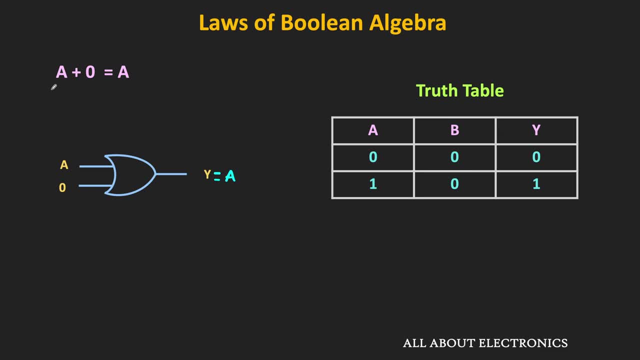 this y is equal to a. That means this: a plus 0 is equal to a. Then the next is the a plus 1 is equal to 1.. That means the OR operation of the a and the logic 1 is always equal to 1.. 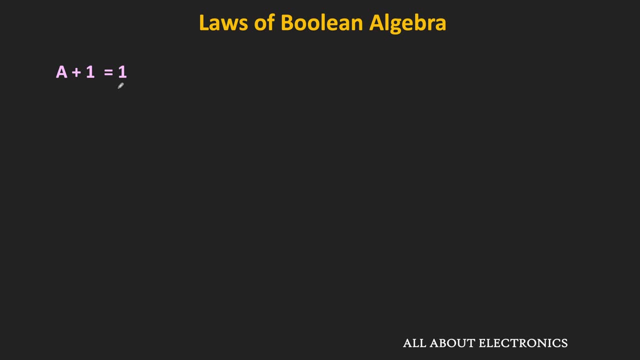 So once again, to prove that, let us see the truth table of the two input OR gate. So in this case, one of the input is always set to 1.. So for the OR gate, we know that when one of the input 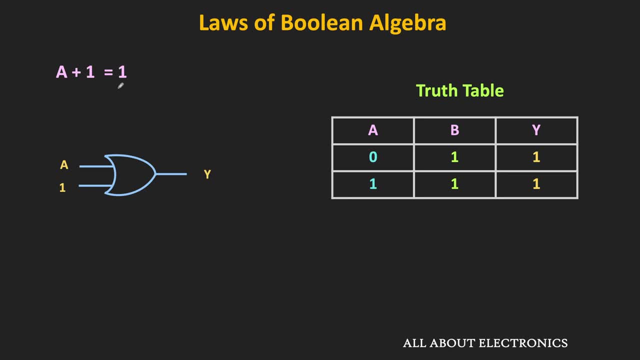 is 1,, then the output is always equal to 1. And therefore, irrespective of the value of a, the output y will always remain 1.. That means this a plus 1 is equal to 1.. Then the next is the a plus a. 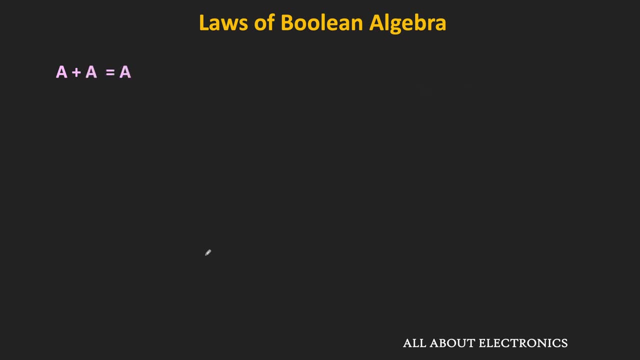 So in the next case, if some gate is a plus 0, then the output b is equal to a. That means during the OR operation, if the both inputs are same, then the output is same as the input, And it is even valid for more than two inputs. So to prove that once again, let us see the 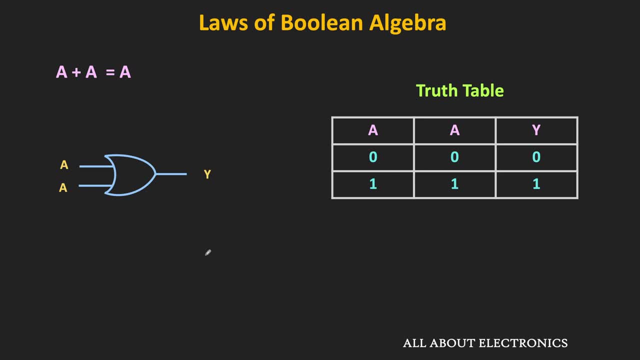 truth table of the two-inputs OR gate. So in this case this b is also equal to a. So here for the: And in that case this output Y is equal to 0.. And when the input A is equal to 1, then the both inputs are 1.. 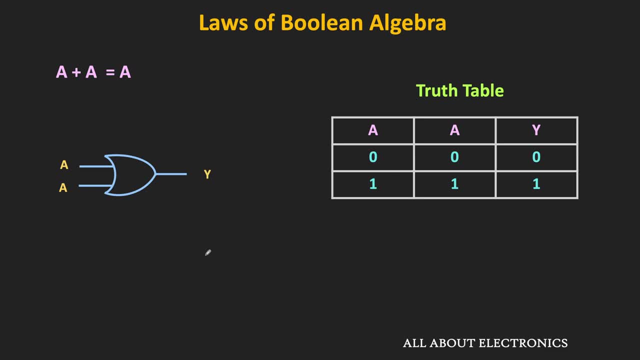 And in that case this output Y is equal to 1.. So, as you can see, the output Y is same as the input A And therefore this Y is equal to A. That means this: A plus A is equal to A. 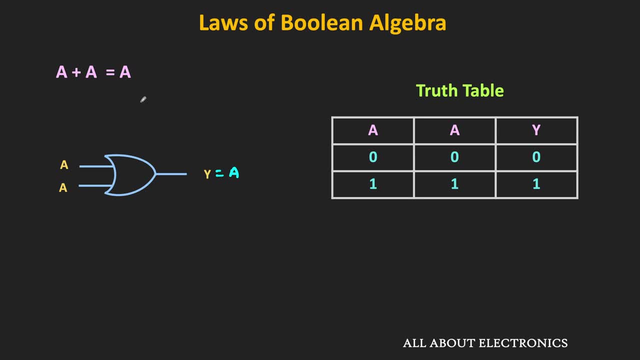 And, as I said, it is also valid even for more than two inputs. That means if we have this A plus A plus A, then that is also equal to A. Then the next is this: A plus A bar is equal to 1.. 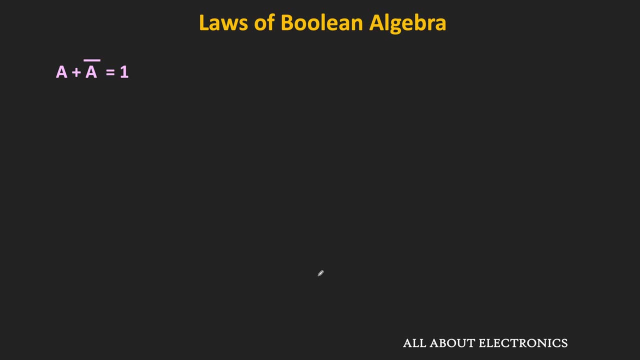 That means the OR operation of the A with its complement is equal to 1.. So once again to prove this expression, let us see the truth table of the two-input OR gate. So in this case this second input is equal to A bar. 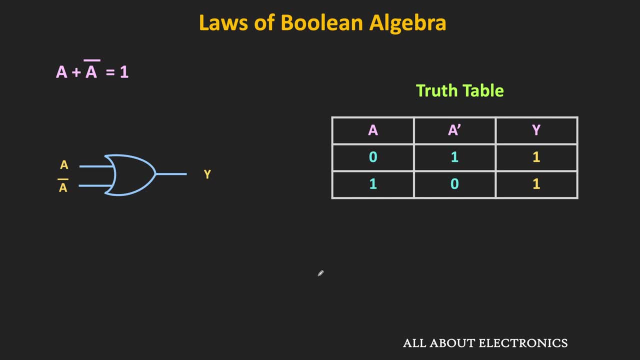 That is the complement of the input A. So here for the input A there are only two possibilities. So when the A is 0, then this A bar is equal to 1.. And whenever this A is 1, then the A bar is equal to 0.. 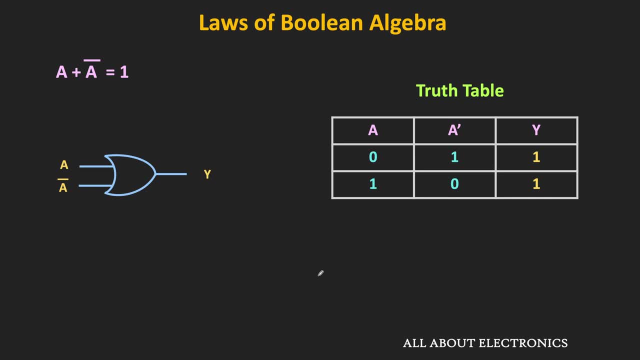 So in both case at least one input is 1.. And we know that for the OR gate when one of the input is 1, then the output will be equal to 1.. That means in both cases this output Y is equal to 1.. 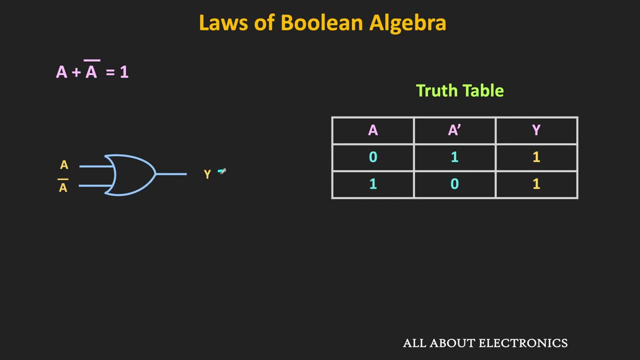 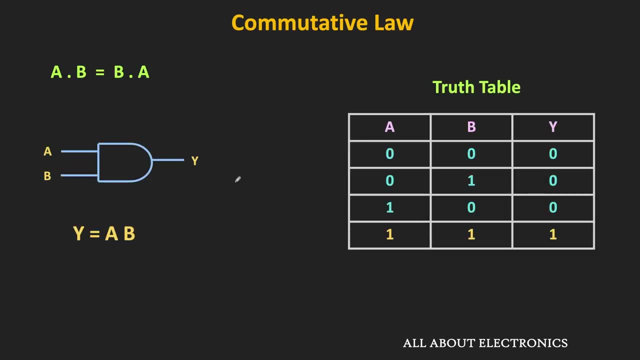 And therefore we can say that For this expression, this Y is equal to 1.. Then the next is the commutative law, which says that the order in which the inputs are connected to the AND gate doesn't matter. For example, if we connect this input B at the top and this A is connected to the bottom, 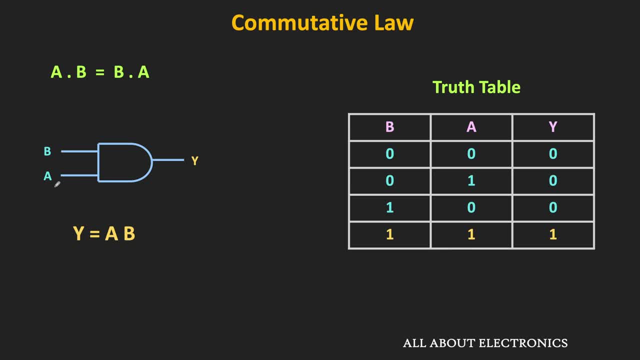 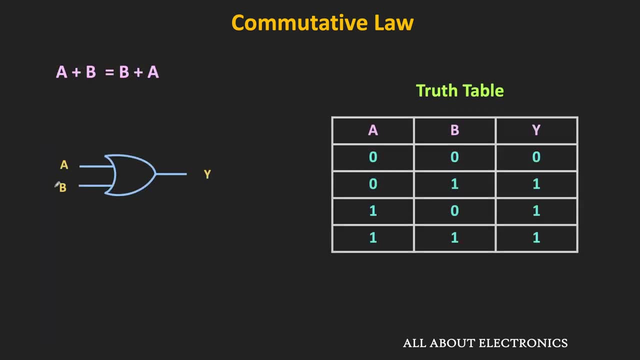 then also we will get the same result. That means this: A dot B is same as the B dot A, And the same is true for the OR gate. That means B is connected at the top and the A is connected at the bottom. 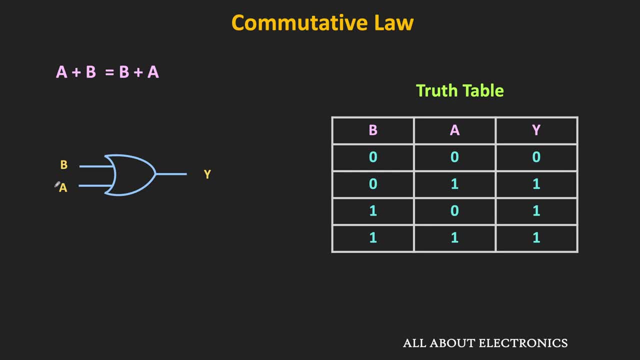 Then also the output of the OR gate will remain same. So that is the commutative law. Then the next is the associative law. So as per this law, the AND operation of the A and B followed by the C is same as the AND. 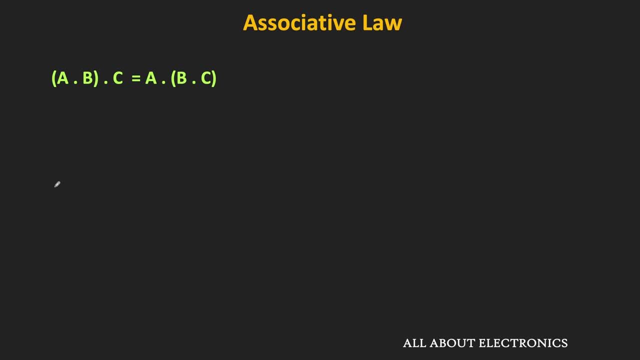 operation of the B and C with the A. So let's say the A and B is ANDed first and then the output is ANDed with the C. Let's say So this output is equal to Y. Now we will get the same result if B and C is ANDed first and then its output is ANDed. 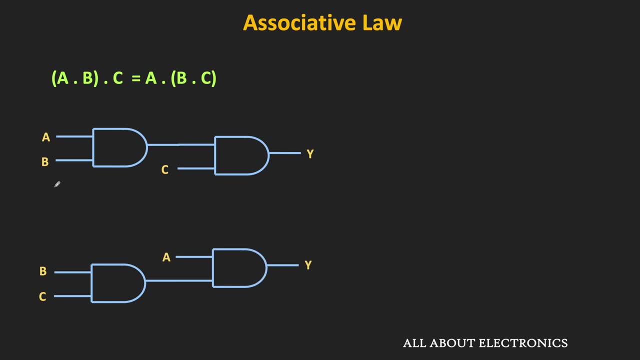 with the A. That means the AND operation of the A and B with the C is same as the AND operation of the B and C with the A, And this can be proved with the help of the truth table. So let's say the output of this A and B is equal to P and the output of this B and 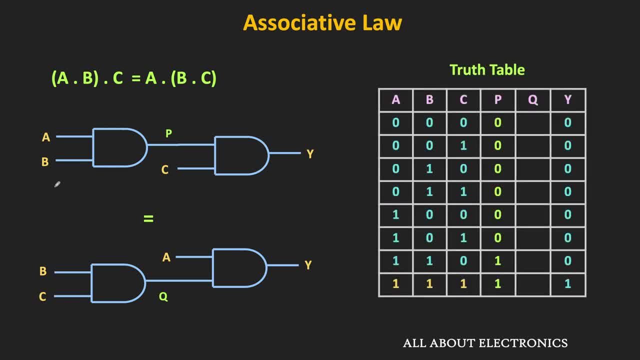 C is equal to Q. So let's say So. let's say This: P will be high when the both inputs, A and B, are high. So now these P and C are ended, So its output will be high when both P and C are high. 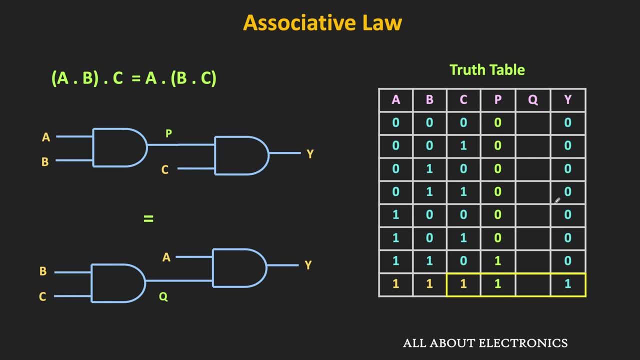 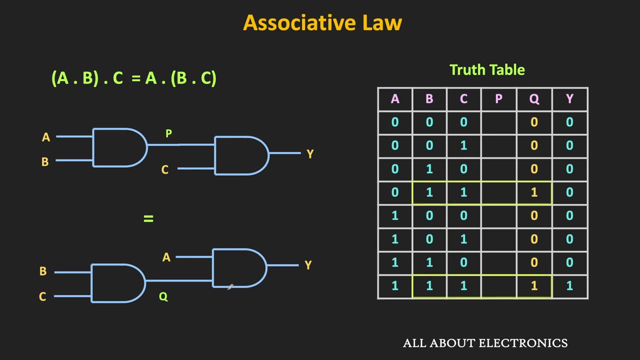 And that is happening only in the last possibility. So this is the output, column Y. Similarly, now let us find the Y for the second circuit, And first let us find this Q. So this Q is high when both B and C inputs are high. 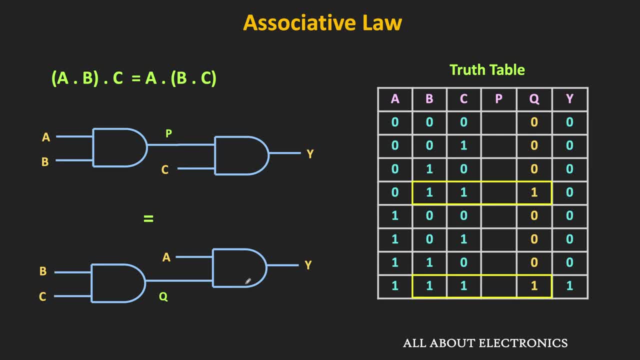 So now this Q is ended with A And once again the end operation of A and Q is high when both inputs, A and Q, are high, And that is happening only in the last possibility. So for the second circuit also, this output column Y, remains same. 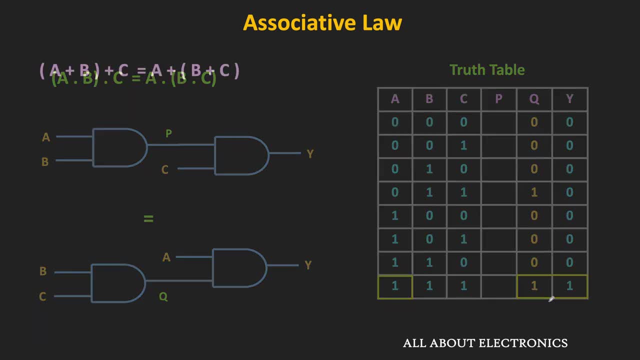 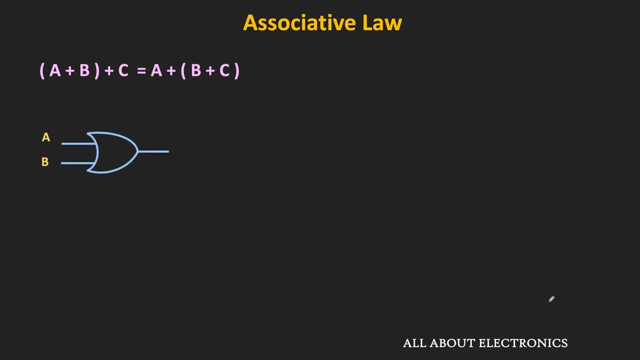 Which proves that both the expressions are same. Similarly, this associative law Is also valid for the OR gate. That means the A or B OR with the C is same as the B or C OR with the A, And it can be also proved with the help of the truth table. 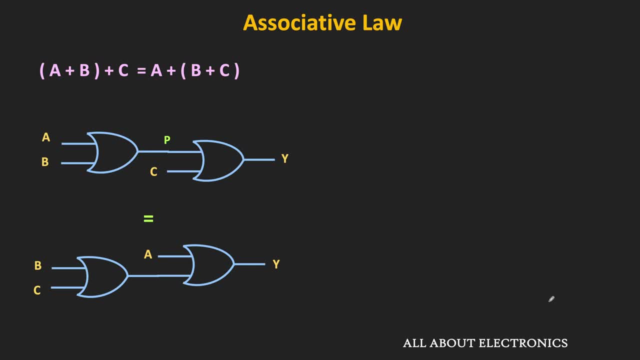 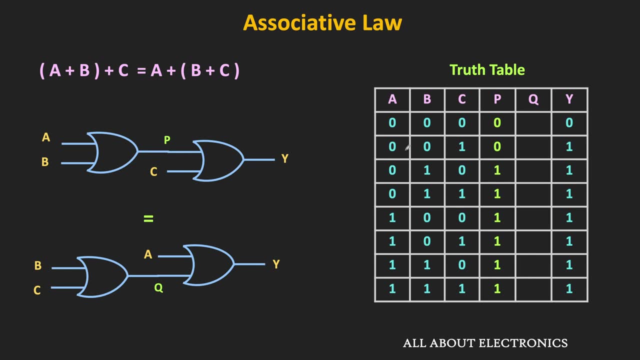 So let's say the output of this A or B is equal to P And the output of this B or C is equal to Q. So now this P is equal to 0 when both inputs A and B are 0. Otherwise it is equal to 1.. 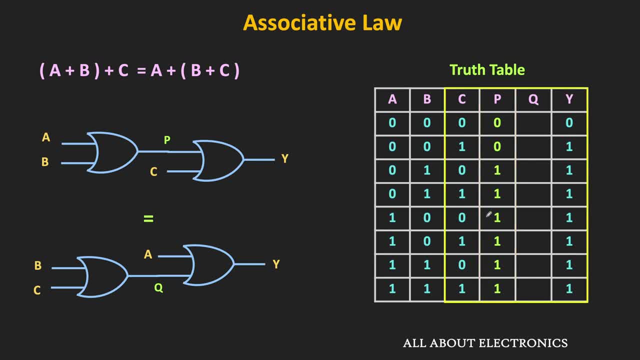 So now let's find this Q. So now this P is equal to 0 when both inputs A and B are 0. Otherwise it is equal to 1.. Now this P is OR with the C, So once again this output Y is equal to 0 when both inputs P and C are 0. 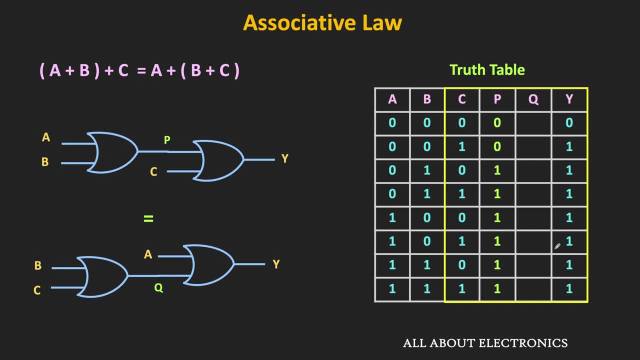 Otherwise this output Y is equal to 1.. So this is the output column Y. Similarly, let us evaluate this Q for the second circuit. So, as you can see, this Q is the end operation of this B and C. That means this Q is high when both inputs, B and C, are high. 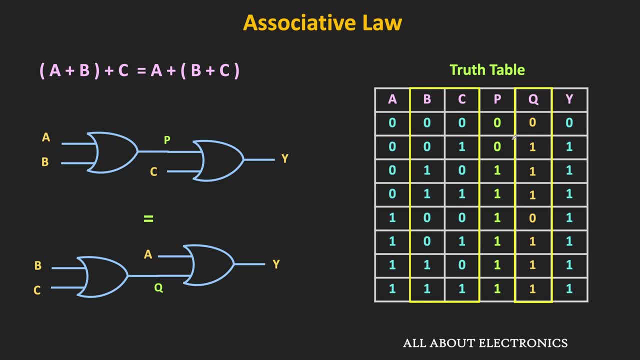 And it is 0 when both inputs B and C are 0.. Now this Q is OR with the A And its output is equal to Y. So this output, Y, is equal to 0 when both inputs A and Q are 0.. 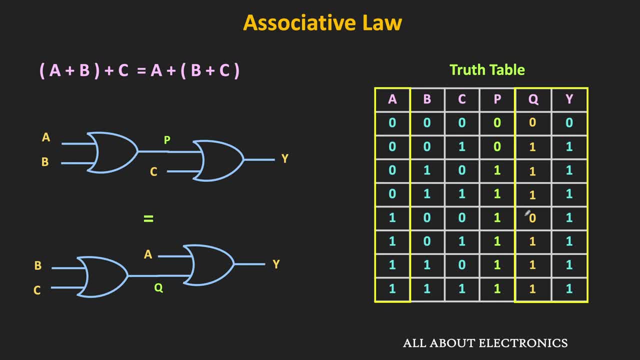 And when any of the input is high, then the output Y is equal to high. So, as you can see, for the both expressions or for the both circuits, this Y column is same, Which proves that both these expressions are the same. So that is the associative law for the AND and the OR operation. 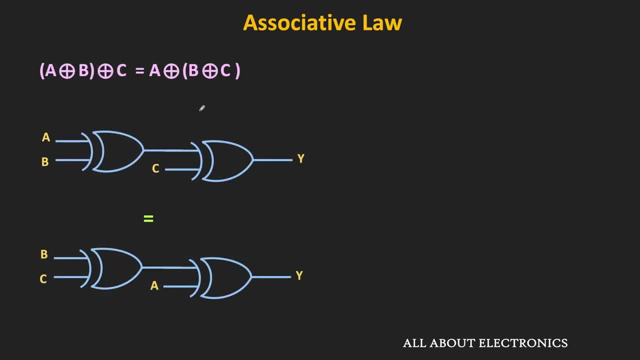 Similarly it is also true for the XOR and the XNOR operation. That means the XOR operation of the A and B with the C is same as the XOR operation of the B and C with the A, And the same is also true for the XNOR operation. 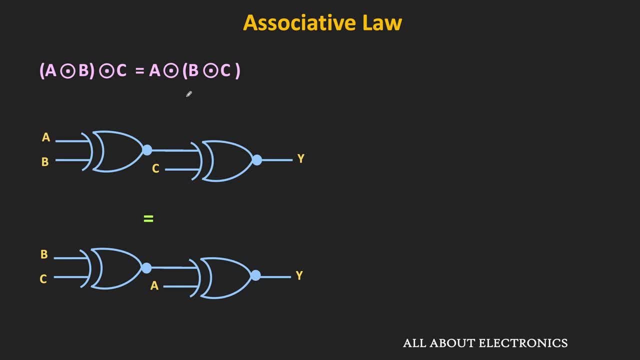 And in fact in the previous video of the XOR and the XNOR gate we have already seen that That means these XOR and the XNOR gates are also associative. So let's see how it works Now. if we talk about the NAND and the NOR gate, then they are commutative, but they are 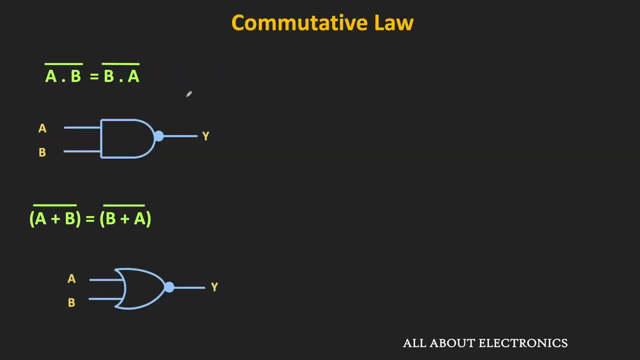 not associative. That means in the NAND and the NOR gate if we interchange the two inputs, then also we will get the same result, But they are not associative. For example for the NAND gate the NAND operation of the A and B followed by the C is not the 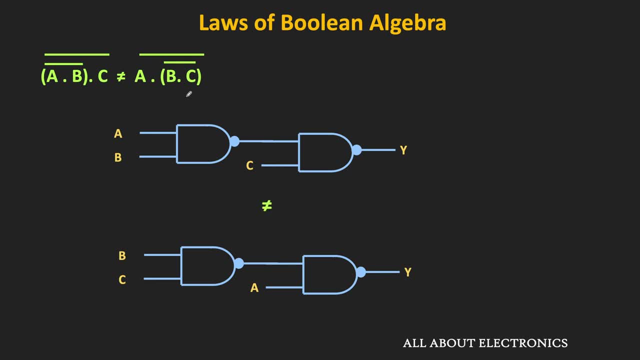 same as the NAND operation of the B and C followed by the A For the NOR gate. also, the NOR operation on A and B followed by the C is not the same as the NOR operation of the B and C followed by the A. That means these NAND and NOR gates are commutative but they are not associative. 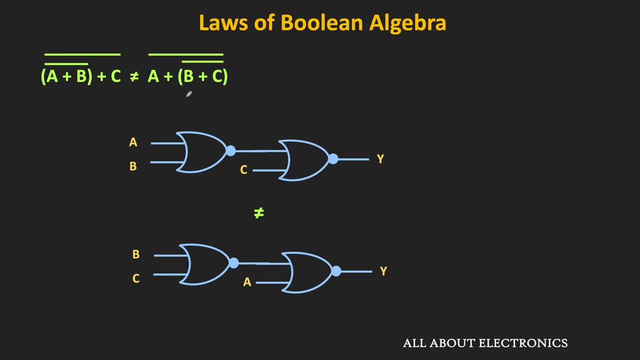 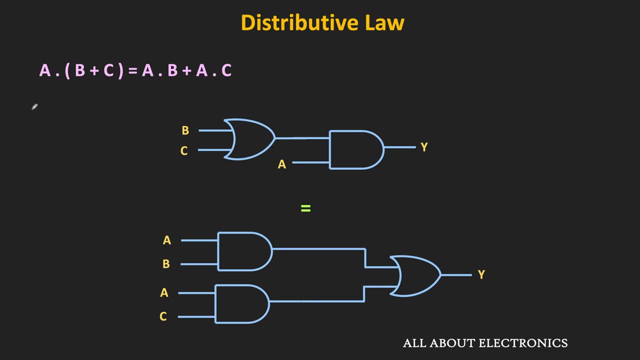 And this can be proved using the truth table. Alright, so now let's move to the next law, that is, the distributive law. So, as per this law, the NAND operation of this A and the B or C is same as the XNOR. 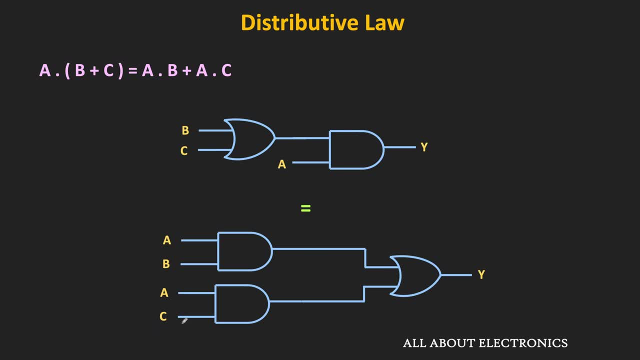 operation of this A and B and the A and C. So basically this law is very similar to our normal algebra, where the variable outside the bracket is multiplied with the East term in the bracket. So here the variable outside the bracket gets ended with the East term inside the bracket. 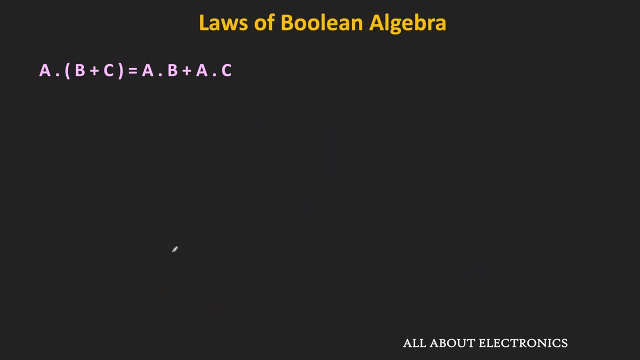 Now this law is also true for more than one variable. For example, the AND operation of this AB with the C or D is same as the OR operation of this ABC and the ABD. That means the variable outside the brackets gets ended with the East term inside the bracket. 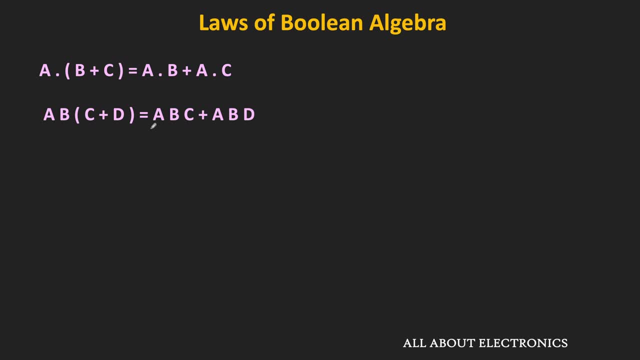 Or if we think other way around, then anything which is common in both terms can also be taken outside as a common term. For example, this A plus AB is equal to A, So in this case this A is common in both terms. 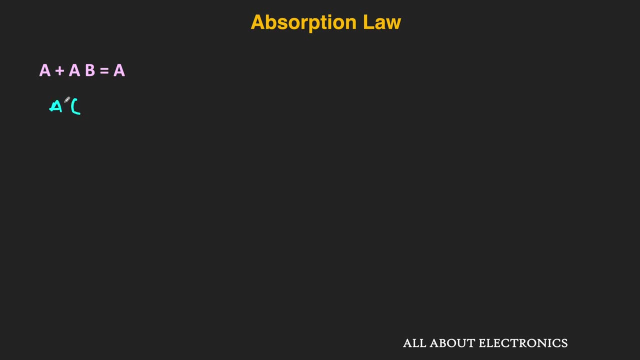 So if we take this A outside, Then we will have This A and 1 plus B. Now we know that 1 plus something is always equal to 1.. That means this term will become 1.. That means now we will have A dot 1 and that is equal to A. 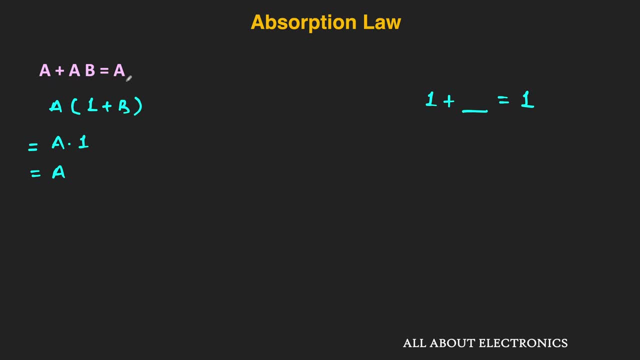 That means this: A plus AB is equal to A. Similarly, the second distributive law is: A plus BC is equal to A plus B and A plus C. So to prove that, let's take the RHS. So, similar to our usual algebra, the each variable gets ended with the other variable. 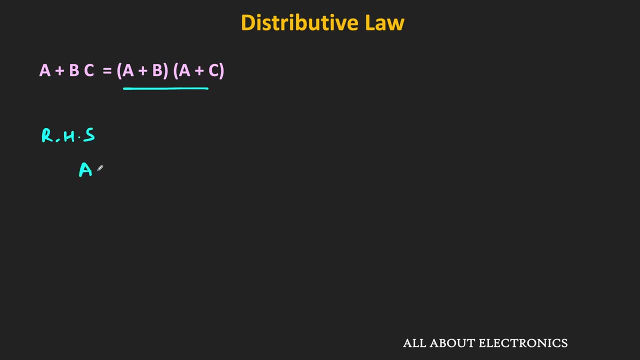 So in this case we can write it as A dot A plus A dot C plus B dot A plus B dot C. Now we know that this A dot A, or the AND operation of A and A, is equal to A And this. 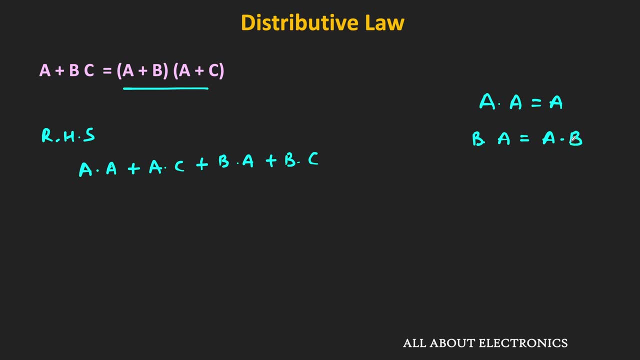 This ba can also be written as ab. That means we can write this expression as a plus ac, plus ab plus bc. So in these first three terms this a is common. So if we take this a outside, then we will have 1 plus c plus b, and this term will remain. 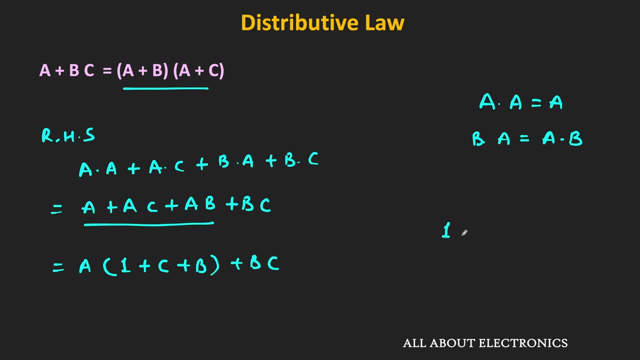 as it is Now. once again, we know that 1 plus something is always equal to 1.. That means this is equal to 1.. So we can write it as this: a.1 plus bc, and we know that this a.1 is equal to a. 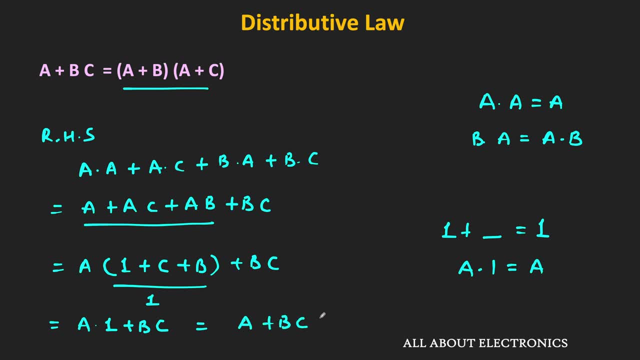 That is equal to a plus bc and that is equal to LHS. So that is the second distributive law. So using the same distributive laws, we can prove that these a and b are common. aa plus b is equal to a, Or in other words, the end operation of the a with a plus b is: 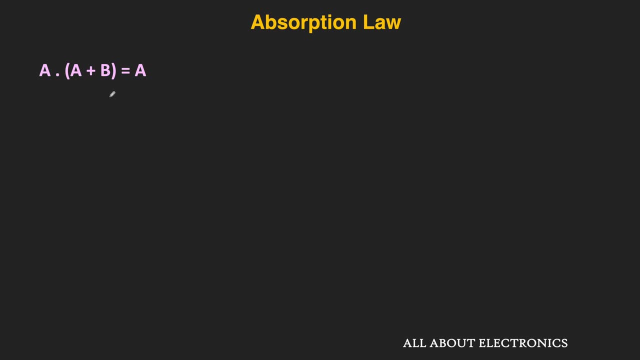 equal to a. So to prove that, let us take the LHS. So here this a will get ended with the isterm inside bracket. That means we can write this expression as aa plus ab. Now, as we have seen earlier, this aa is equal to a. That means we can write this expression: 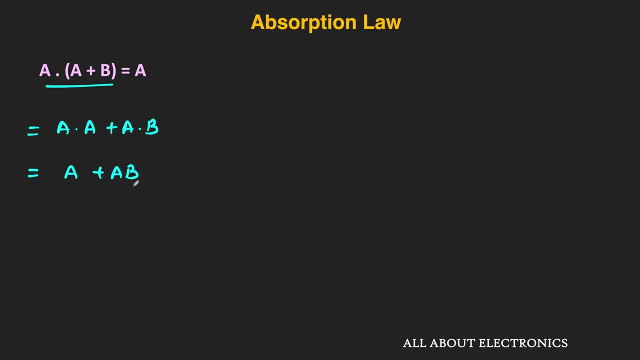 as a plus ab, And we have just seen that this aa plus ab is equal to a. That means the is equal to a. So this is how, using this Boolean laws, it is possible to minimize the Boolean expressions. So at the end, now let us look at the double negation. So we know. 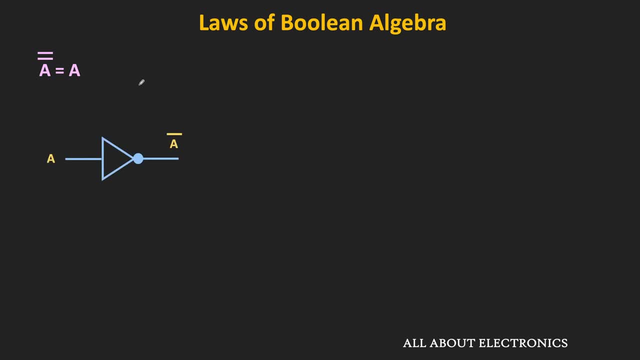 that the complement of the a is equal to a bar, And if we once again take the complement of this a bar, Then it will be equal to A double bar. So if A is equal to 1, then its complement, A bar, will. 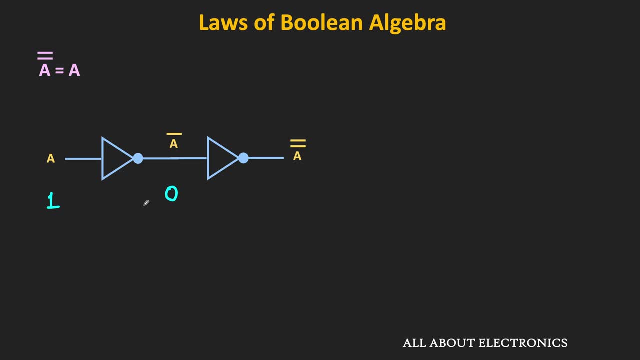 be equal to 0. And once again, if we take the complement of this A bar, then it will be equal to 1.. So if you see this A double bar, then it is same as the A. That means the complement of the A bar is same as the A. So in this way we have covered most of the Boolean laws.